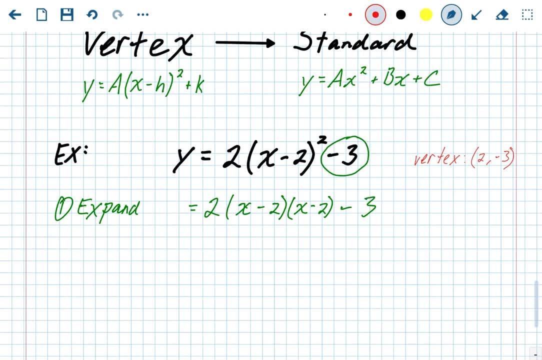 All right, so we expanded. Now we're going to FOIL. Okay, so we're going to FOIL. We have a binomial times a binomial. It's going to be a perfect square trinomial. So some of you know the pattern, so you don't have to do the full FOIL. 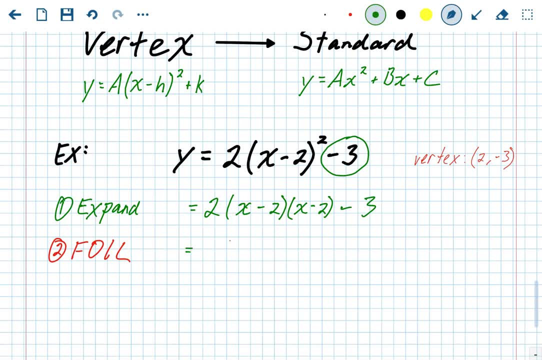 but I'll do the full one on this first problem, That 2 again is just going to stay out front and that minus 3 is going to stay out back. Okay, do not forget those parts. All right, and then the FOIL: first outside, inside, last. 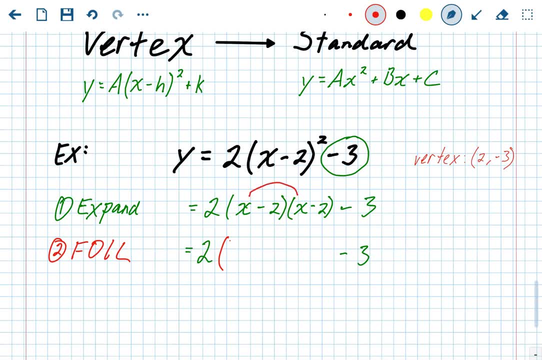 It's going to give us x squared x times x, x squared Outside, inside last, All right, Inside negative 2x, inside negative 2x, and then last negative 2, and negative 2 is plus 4.. 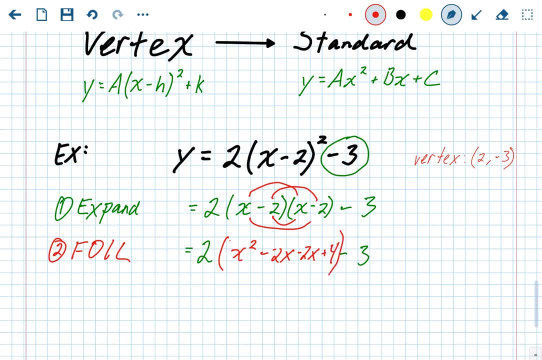 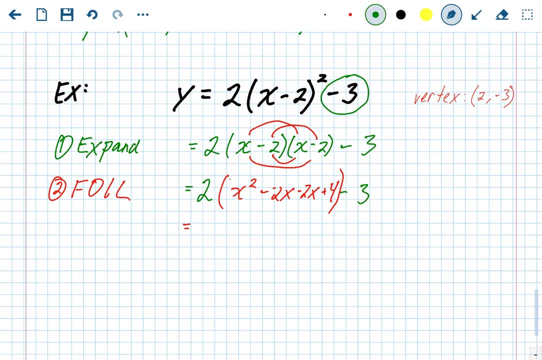 Okay, Combine like terms on the inside. So again, the 2 is just going to hang out front. Combine like terms: x squared minus 4x. Okay, All right, so we're going to FOIL. We're going to FOIL. 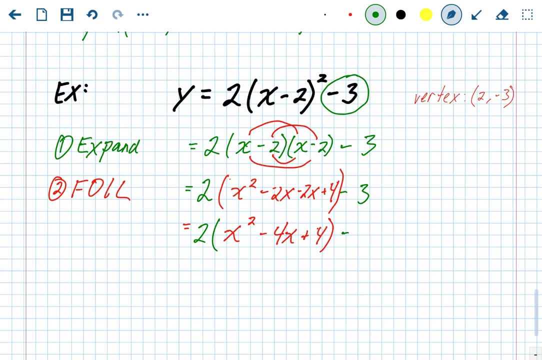 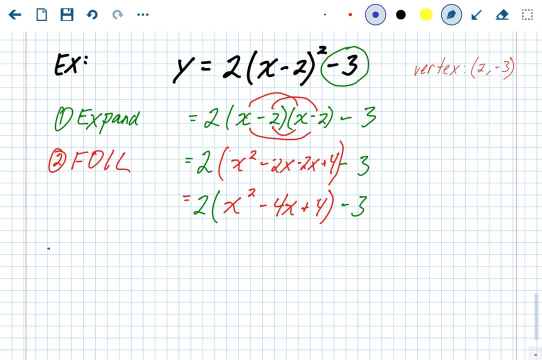 It's going to be like this: It's going to be 1 plus 2, plus 4.. And then again the minus 3 at the end. All right, Your next thought is probably correct: You're going to want to DISTRIBUTE. 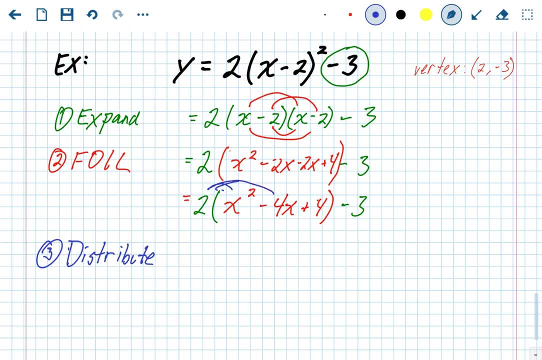 Distribute the 2. that's out front. Okay, Now, when you distribute the 2,, you can only distribute it until the parentheses end. So you're going to take the 2, and you're going to multiply it times the trinomial, but not times the 3 at the end. 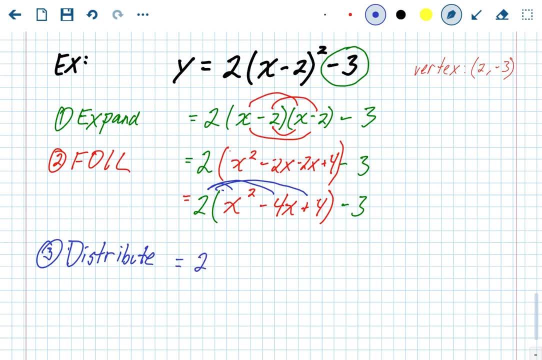 All right, Perfect. so 2 times x squared is 2x squared. 2 times negative, 4 is negative 8x. 2 times positive, 4 is positive 8. and then that minus 3 does not get multiplied, you do not distribute to it, it just stays out back. 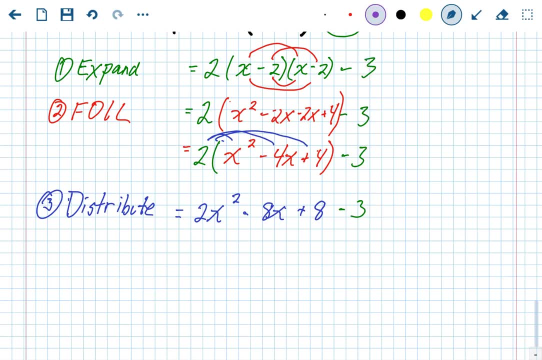 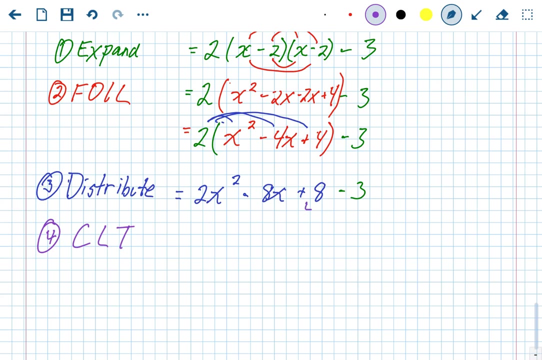 alright, almost done. last step here is to just combine like terms. finally, that negative 3 is going to come into play when we combine like terms: CLT, alright. so what we're combining is we're combining those two numbers of that variable at the end: plus 8, minus 3. 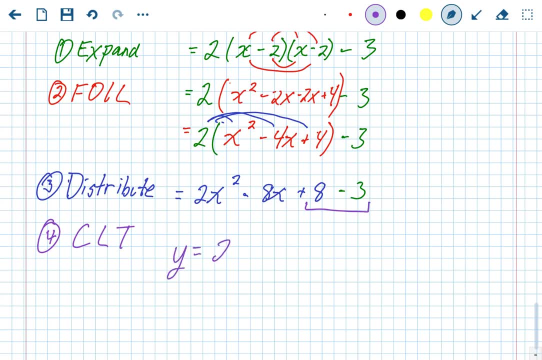 that's going to give us: y equals 2x squared minus 8x, and then 8 minus 3 is plus 5, which is in standard form. make sure your a value didn't change. the a value in standard form is a 2. 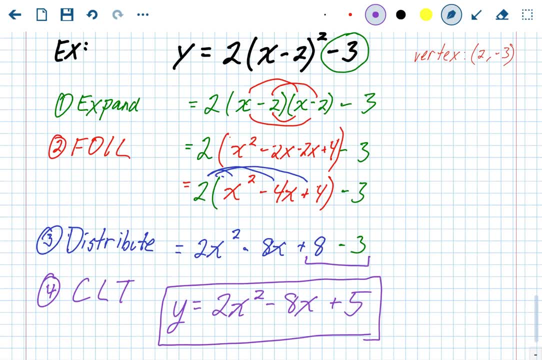 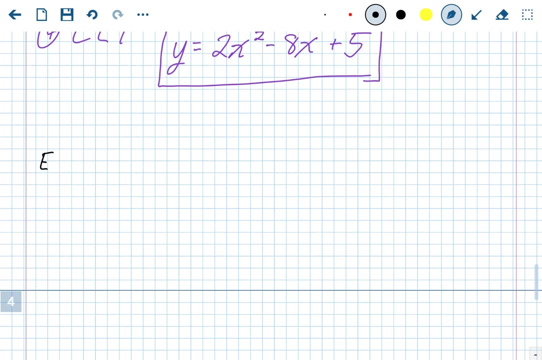 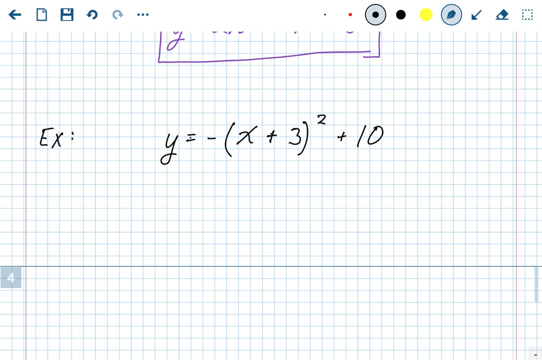 the a value in the original problem was also a 2. so vertex to standard: expand, FOIL, distribute, combine like terms. let's do one more. say we have y equals negative x plus 3 squared plus 10- again your vertex. you should be able to find the vertex immediately. 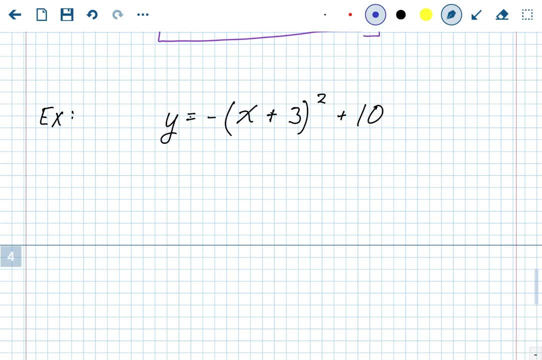 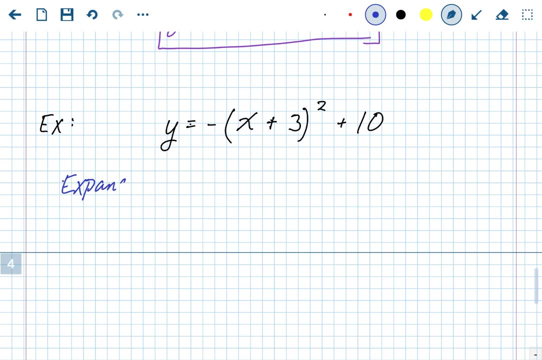 the vertex is negative: 3, 10. alright, let's do the four steps. start with expand. expand is really rewriting the problem. the negative stays out first. the negative stays out first. so that's where we're at. so let's get started. front, and we're going to write it as x plus 3 times x plus 3 plus 10 stays at the end. 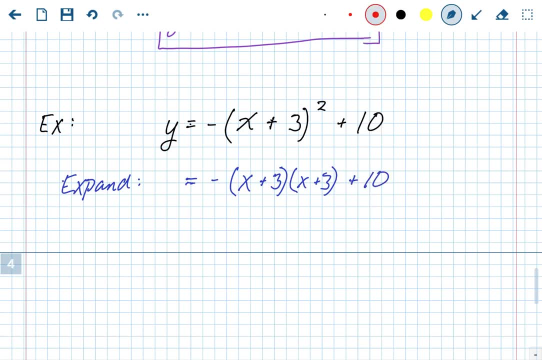 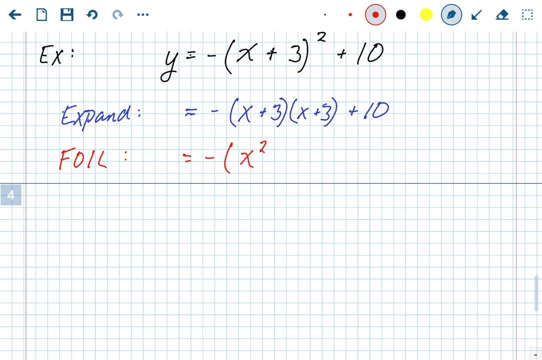 all right. so let's expand foil: first outside, inside, last. again, the negative out front is going to stay out front first, outside, inside, last. for a perfect square, trinomial is going to be x. squared outside and inside are both 3x, so that'll be plus 6x, and then last 3 times 3 is 9. 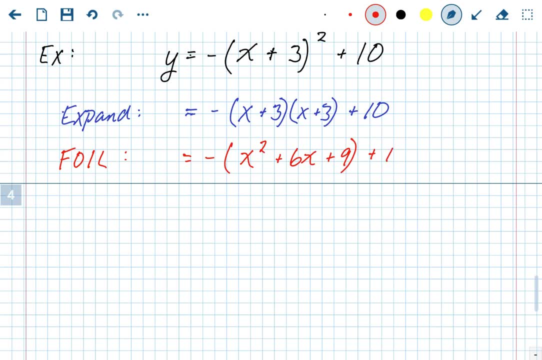 in parentheses. don't forget the plus 10. okay, distribute. there's not a number in front, but there is a negative sign. so we are going to distribute that negative sign. we're going to multiply: Sharpened voting, okay, and then plus 3 times 3. don't forget the plus 10. 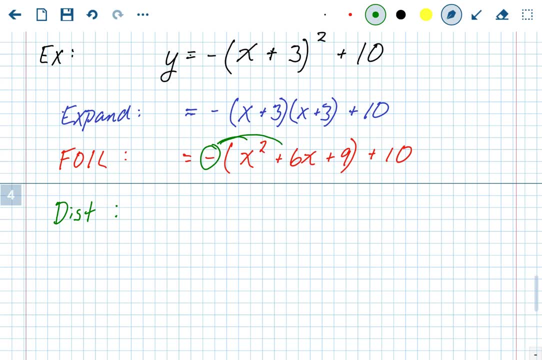 gonna take the negative and again you're basically multiplying by negative 1, which is just gonna flip all the signs. so, instead of positive x squared, it's now negative x squared. instead of plus 6, it's minus 6 and 6x, and instead of plus 9, it's minus 9. right, and now you got the.